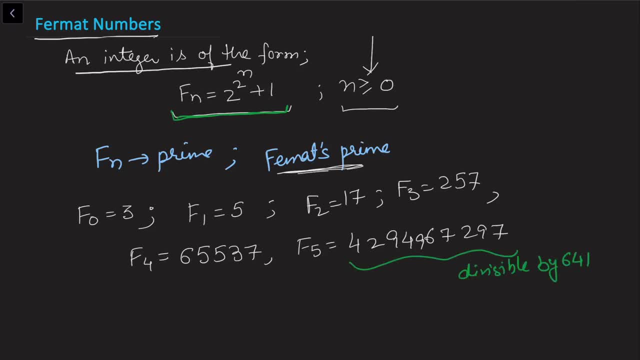 and f5. this is equal to 4294967 and f5- this is equal to 4294967 and f5- this is equal to 4294967 297, and we know that this is divisible by 641. so this conjecture by fermat that this is the 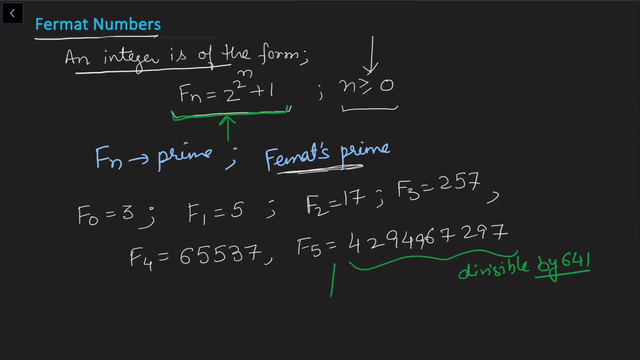 formula for the prime number is not true and as we see that f5 is a composite number, but fermat numbers or the fermat primes numbers are very much in use for the primality testing and which is used a lot in cryptography and in the other areas. so one of the tests which involves these fermat 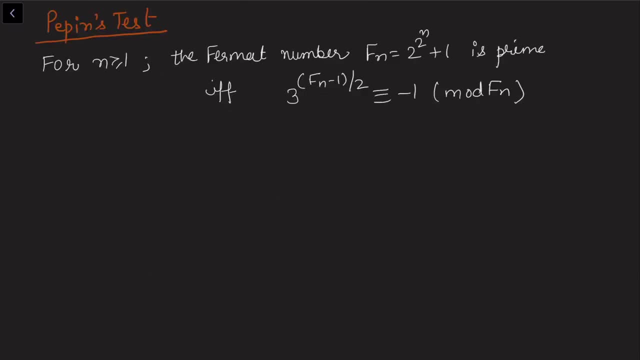 prime number is pepin's test and it says: for n greater than or equal to 1, the fermat number fn which is given by this is prime if, and only if, 3 to the power fn minus 1 by 2 is congruent to minus. 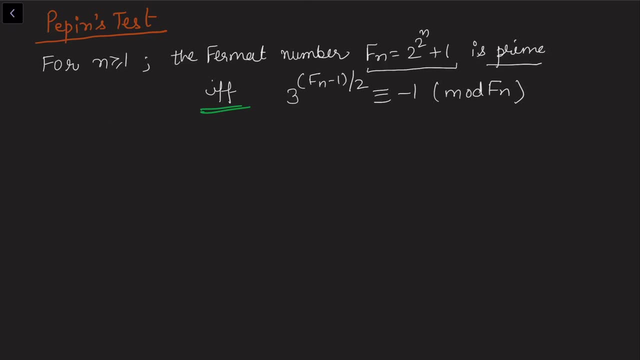 1 modulo fn. now to see this, let's take an example. take f3 and by the formula since i am calculating it, f3. so the value for n here is 3, and this will become 2 to the power, 2 to the power, 3 plus 1. so 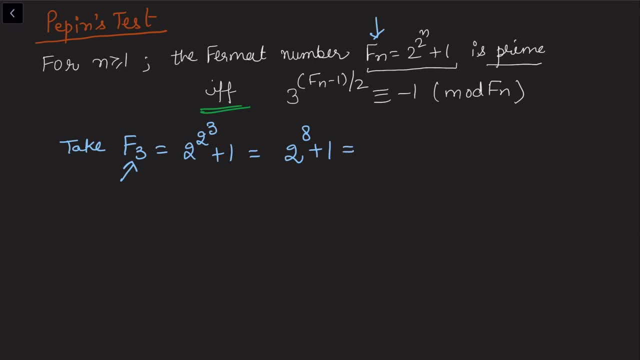 you see that this is 2 to the power 8 plus 1 and that becomes 257. so now let's apply the test. in this case this will become 3 to the power fn. so i want to check now this congruence and if this congruence hold, we. 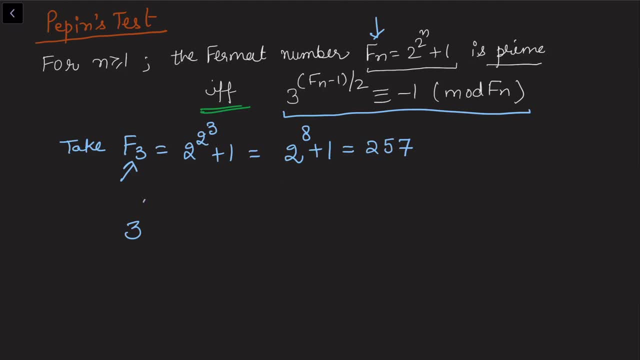 say that f3 is prime, so 3 to the power fn, that is 257 minus 1 by 2, so this will become: this is 3 to the power 128, which is equal to 3, cube 3 to the power 5 and whole raised to power 25, so we can: 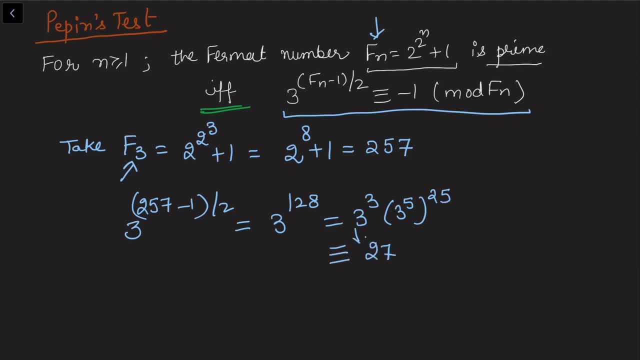 split that by 2 and we get 3 to the power 5 and whole raised to power 25. so we can split that, which is further congruent to 27: 3 cube is 27 and this value 3 to the power 5. this is congruent to: 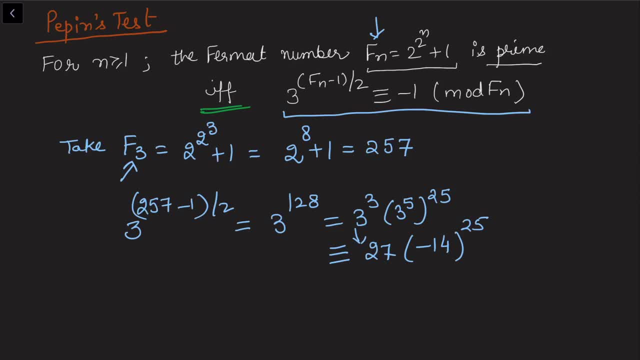 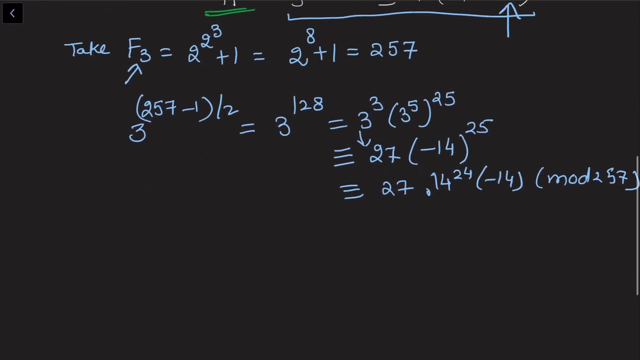 minus 14 and keep the power as it is, that is, 25. this is further congruent to 27 into 14, raised to power 24 multiplied by minus 14. and all this is going in modulo 257, because you can see that here we are taking inside modulo fn. this is further congruent to 27 multiplied by 17, into 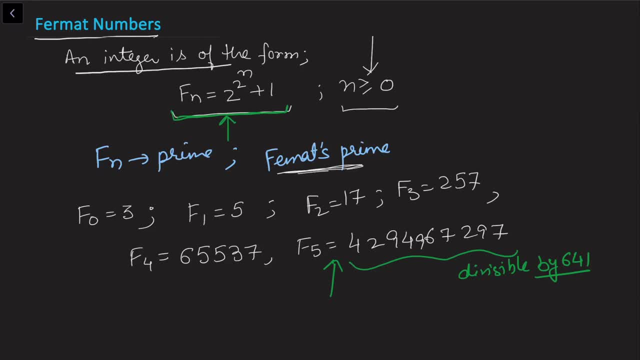 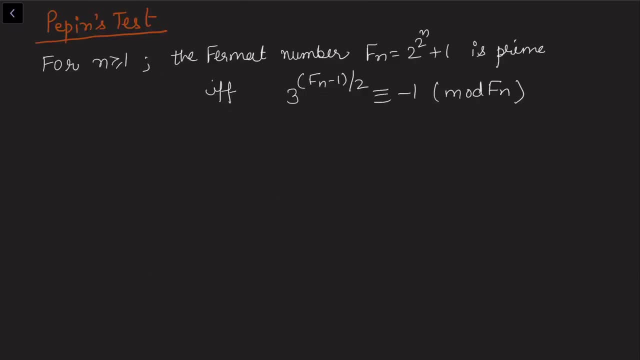 used a lot in cryptography and in the other areas. so one of the tests which involves these fermat prime number is pepin's test and it says: for n greater than or equal to 1, the fermat number fn which is given by this is prime if, and only if, 3 to the power fn minus 1 by 2 is congruent to minus. 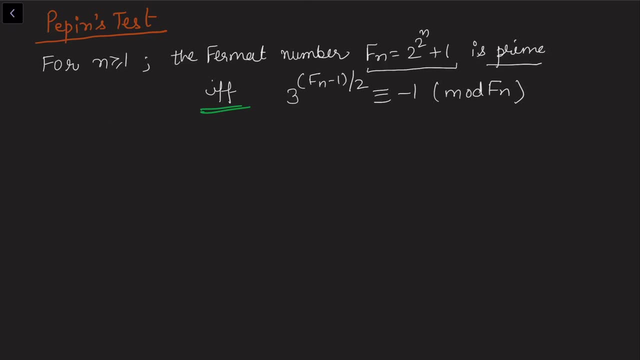 1 modulo fn. now to see this, let's take an example. take f3 and by the formula since i am calculating it, f3. so the value for n here is 3, and this will become 2 to the power, 2 to the power, 3 plus 1. so 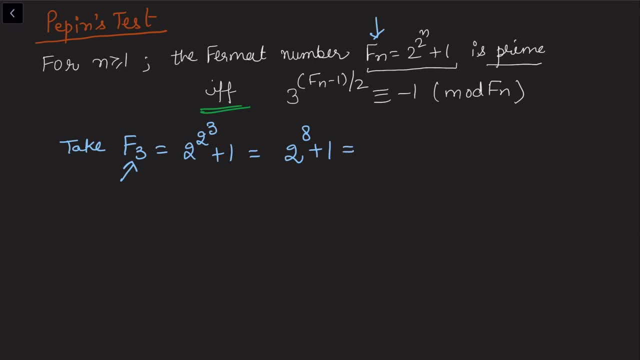 you see that this is 2 to the power 8 plus 1 and that becomes 257. so now let's apply the test. in this case this will become 3 to the power fn. so i want to check now this congruence and if this congruence hold, we. 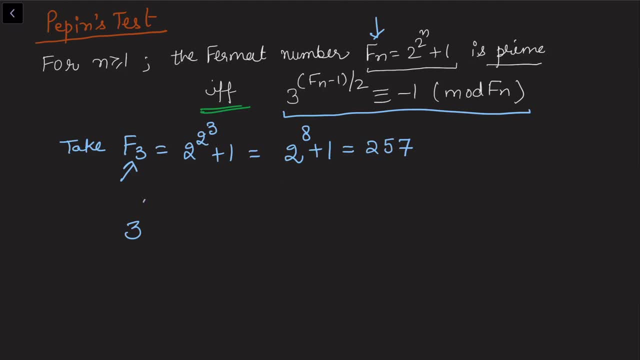 say that f3 is prime, so 3 to the power fn, that is 257 minus 1 by 2, so this will become: this is 3 to the power 128, which is equal to 3, cube 3 to the power 5 and whole raised to power 25, so we can: 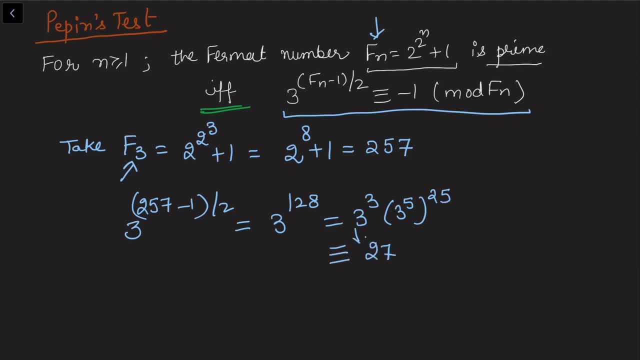 split that by 2 and we get 3 to the power 5 and whole raised to power 25. so we can split that, which is further congruent to 27: 3 cube is 27 and this value 3 to the power 5. this is congruent to: 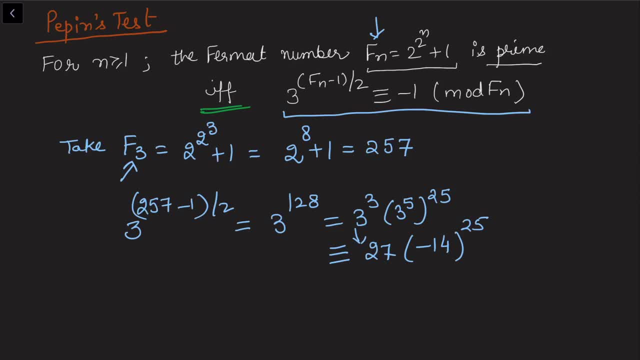 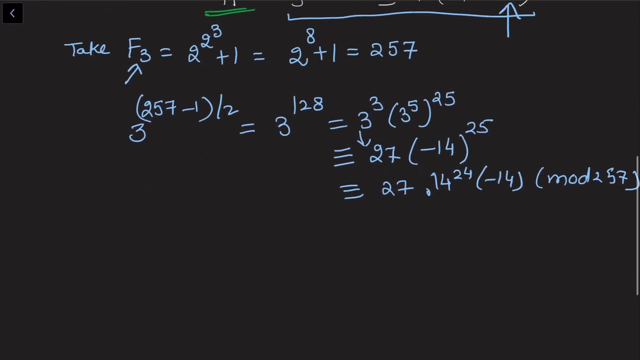 minus 14 and keep the power as it is, that is, 25. this is further congruent to 27 into 14, raised to power 24 multiplied by minus 14. and all this is going in modulo 257, because you can see that here we are taking inside modulo fn. this is further congruent to 27 multiplied by 17, into 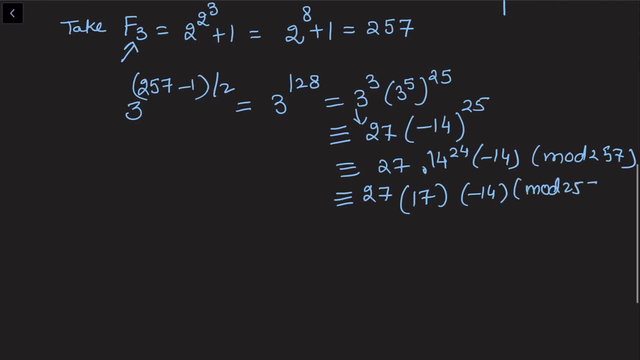 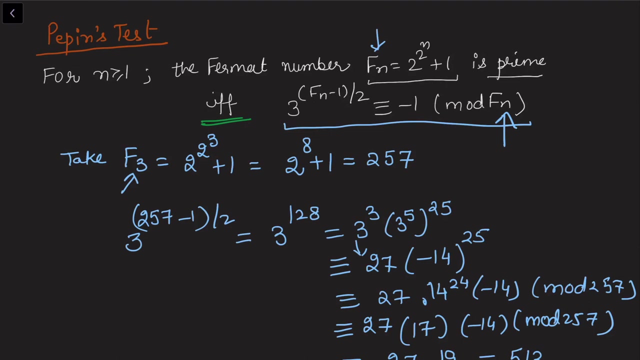 minus 4, with the same condition, modulo 257. this is congruent to 27 multiplied by 19, which is further congruent to 513. 513 is congruent to minus 1 modulo 257, and hence the result hold. look at the result again. we wanted to know. this is to be congruent minus 1, and here we got this.